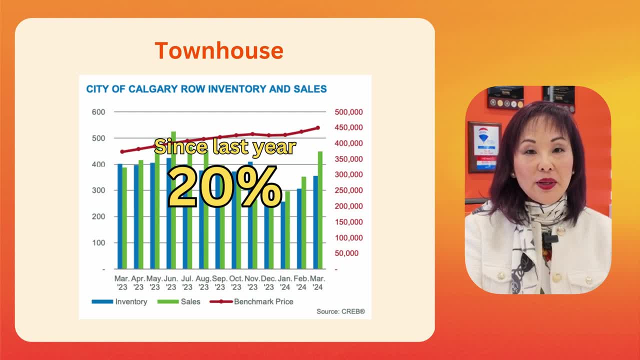 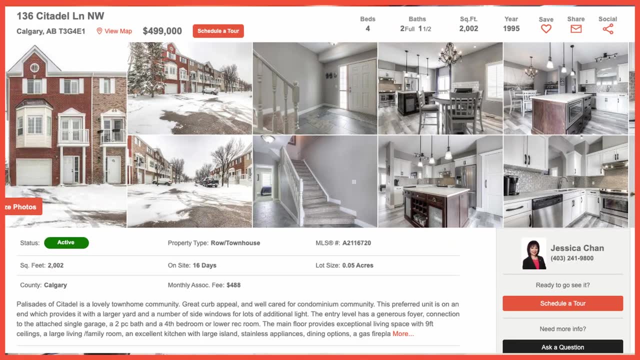 and a 20% increase from March 2023.. This is a very sharp increase in Calgary real estate history. For example, in North Calgary, if you want to buy a townhouse with a single attached garage, you need to pay close to, or over, $500,000. 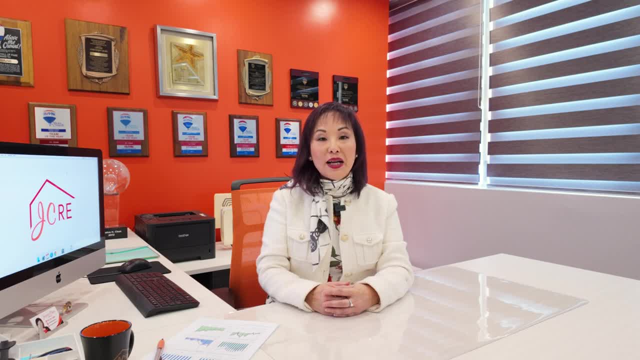 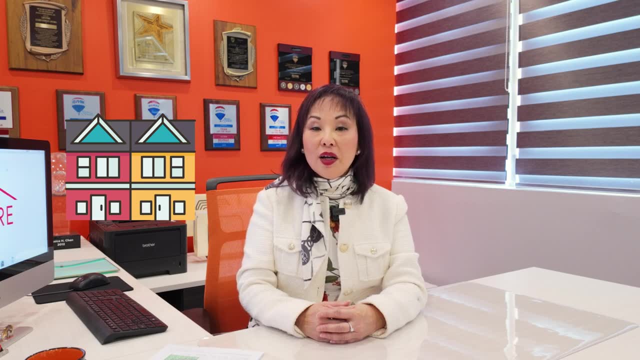 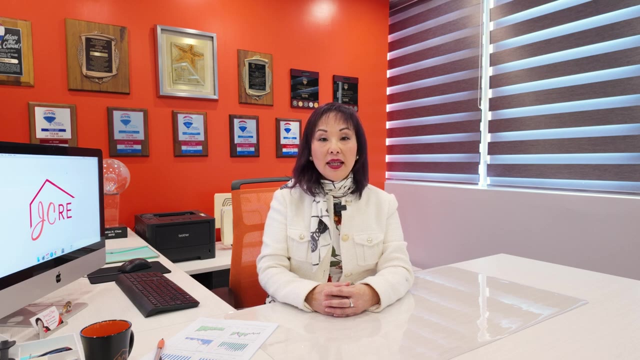 When the similar townhouses were sold under $400,000 one year ago. Lately we sold a few townhouses in Nolan Hill and each time we got 8 to 10 offers. Apartment sales in different parts of Calgary has different trends in the last one year. 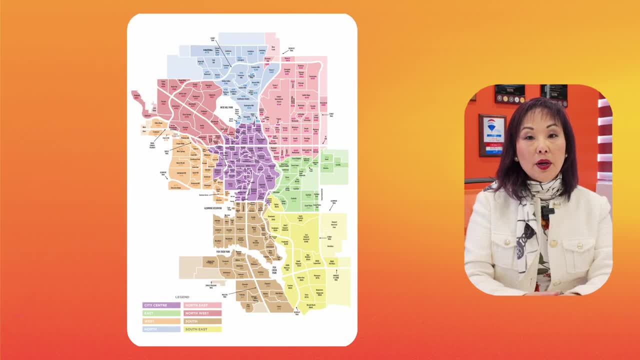 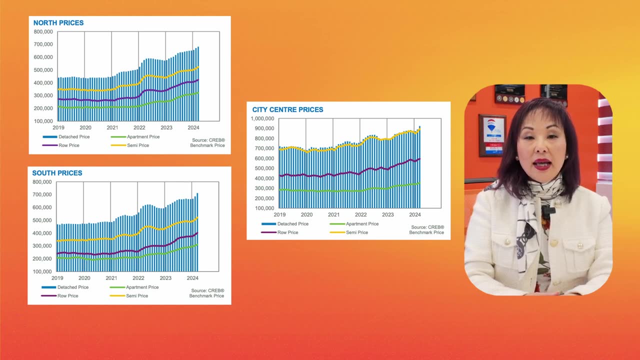 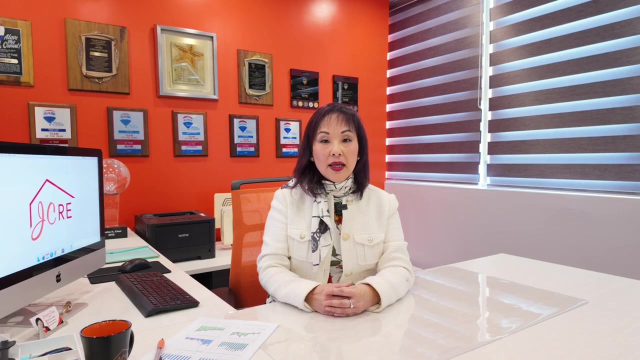 If you take a closer look at the graph in different parts of the city, you will notice that the North and South area, mostly in the newer areas, are selling less And their sale price increase is sharper than in the inner city, especially in the downtown core. This phenomenon is due to the demand in the suburbs. where the newer communities are in high demand. People tend to like the newer communities which have better shopping and other facilities. You will also notice the age group around 60 to 70 years old are ready to downsize to apartments and many of them will not pick downtown areas. 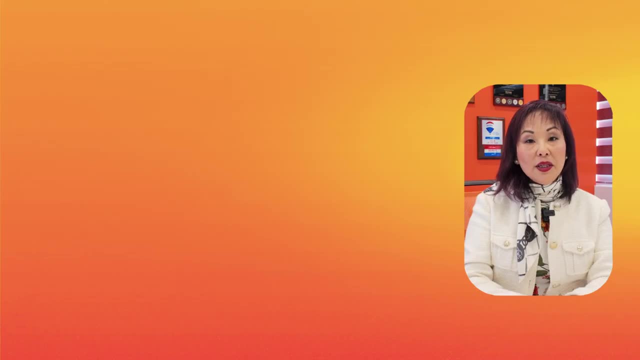 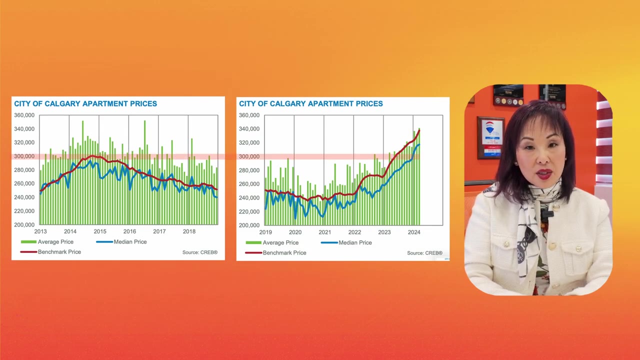 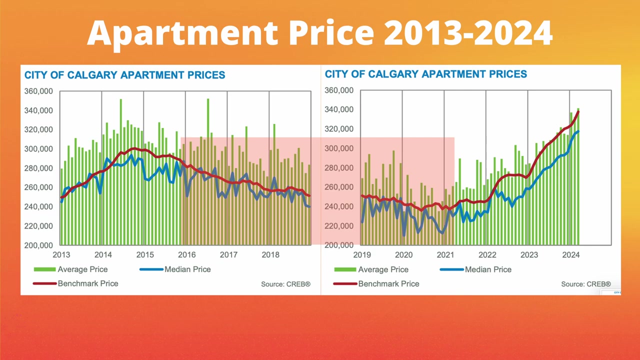 For downtown apartments. some owners bought their units at the peak market in 2014 and still may suffer loss when they are selling at this time. Downtown apartments have dropped significantly during 2016 to 2020 and are still recovering now. If you are interested to know more about the downtown market situation, 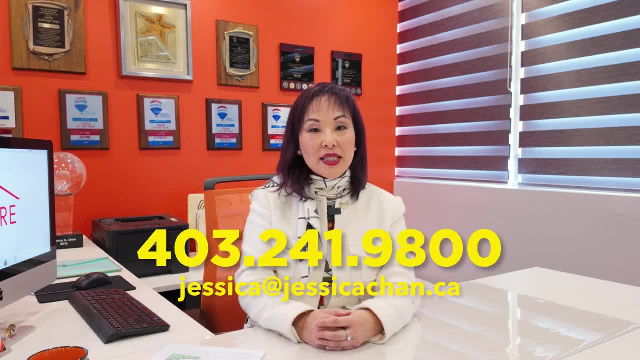 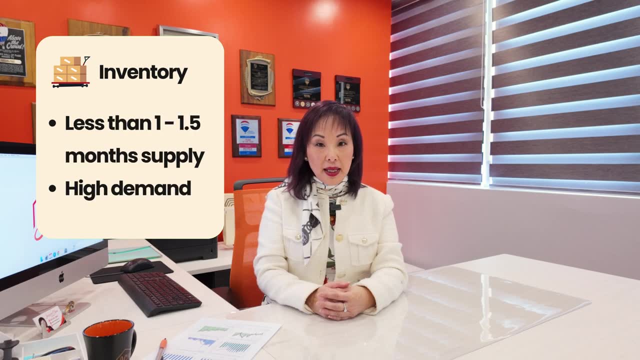 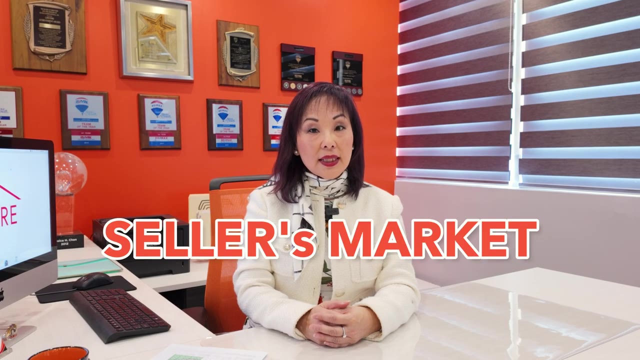 please feel free to call or email me to discuss. In terms of inventory, we are still low. In many areas there are less than one month's supply or may have only one and a half month's supply. That is also the main reason the seller's market condition continues. 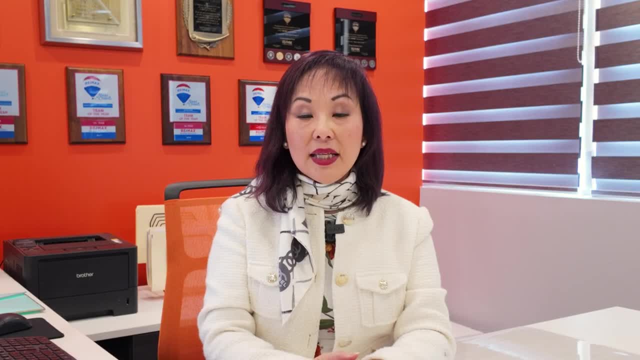 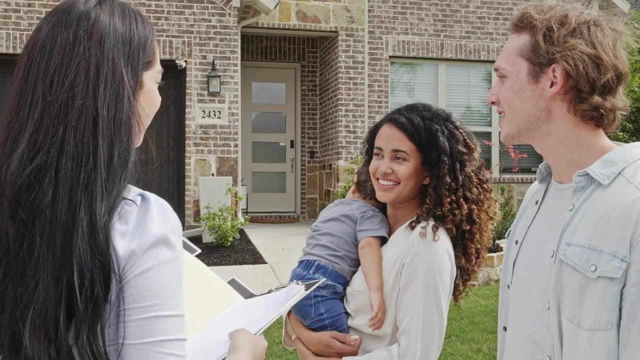 Despite the high interest rates, the demand in real estate is still strong in Calgary. We are expecting the Bank of Canada to lower the lending rate in June and will continue to increase the demand in Calgary, And that might help more buyers afford to buy. 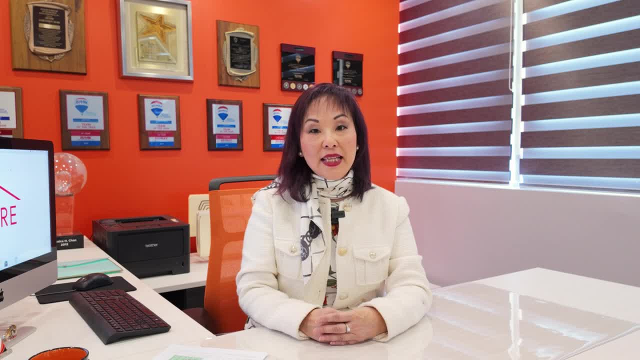 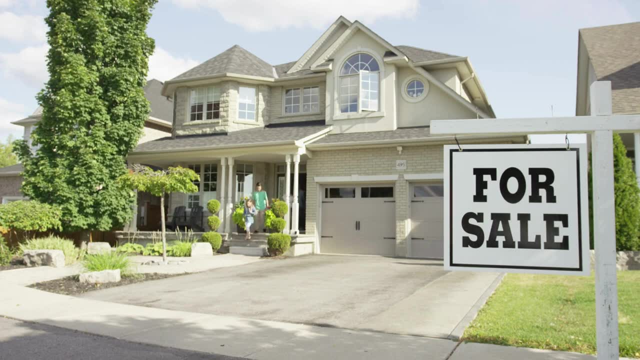 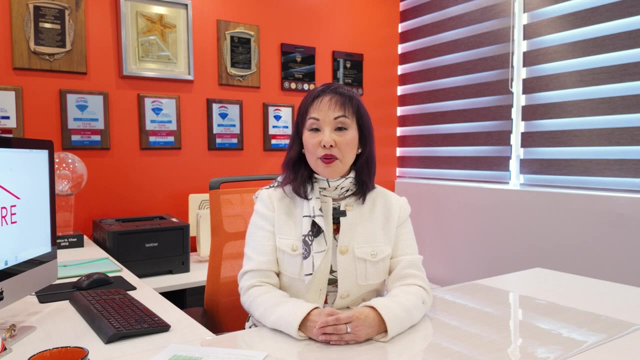 We have good confidence. the market will remain strong and steady in Calgary throughout this year. If you are the homeowner planning to sell this year with this uptrend market, you need a good, experienced agent who can give you the most current market value and help you to get the top-notch dollar for your property. If you are the homebuyer searching for your dream home in this confusing market, the last thing you want is to pay way over this price and find out later that you are paying too much during competition. You need an honest and experienced agent to offer you the strategic way to compete.